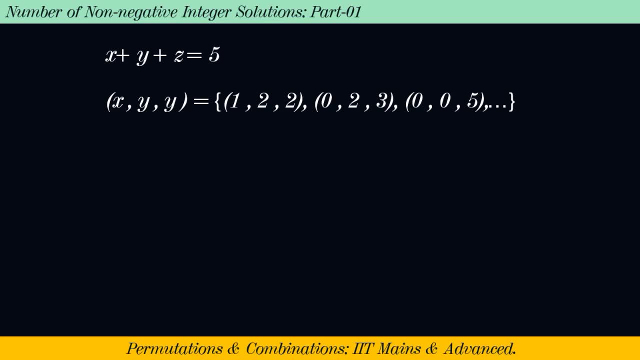 2,, 3,, 0,, 0,, 5, because their sum is equal to 5.. Hence they are solutions of the equation: x plus y plus z is equal to 5.. But there is a big challenge here. Can we find the numbers of all such ordered triplets, or? 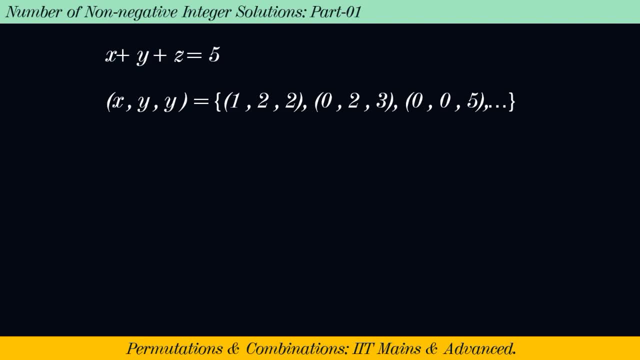 solutions without actually writing them. Actually, it is difficult to answer at this moment, but there must be a way to answer it. Let us adopt some convention here to get our answer. Suppose each blue ball represent natural number 1 and each yellow colored ball represent natural 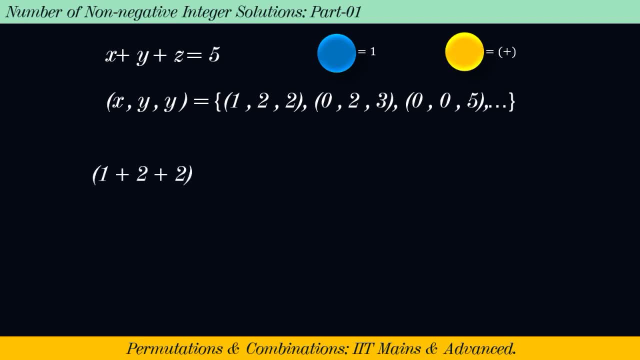 sign of addition. Then 1 plus 2 plus 2 can be interpreted as sequence of 1 blue ball, 1 yellow ball, 2 blue ball, 1 yellow ball and 2 blue ball. Similarly, 0 plus 2 plus 3 can be interpreted as a sequence of no ball, 2 blue. 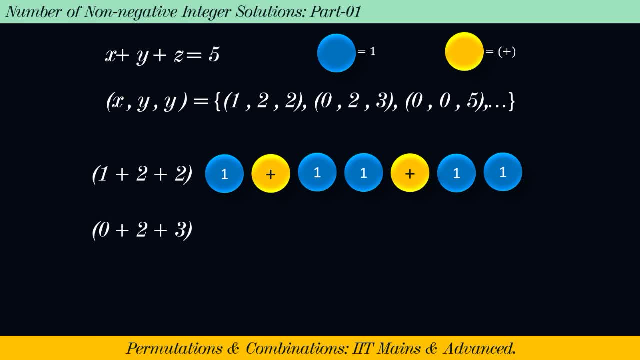 Zero plus two plus three can be interpreted as a sequence of no ball yellow ball, two ball yellow ball and three blue colored balls. Similarly, zero plus zero plus five can be represented as a sequence of no ball yellow ball, no ball yellow ball and five blue colored balls. 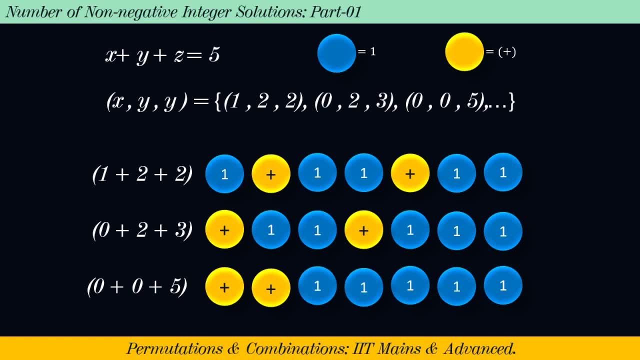 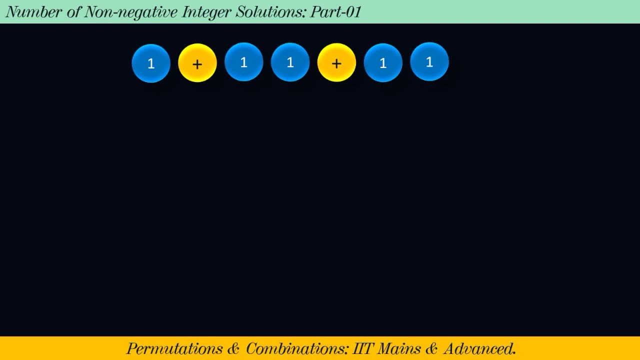 Please note that if no blue colored balls are found adjacent to yellow colored ball, then no ball or zero ball to be assumed on either side of yellow colored ball. Now the question may arise: why are we doing this? Actually, each arrangement of five blue colored balls and two yellow colored balls give us a non-negative integer solution to equation. x plus y plus z is equal to five. 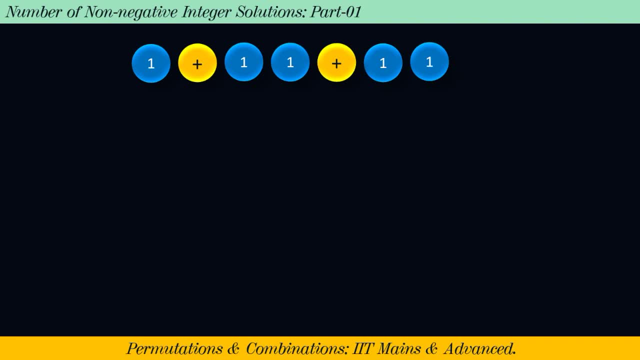 And the good news is we know how to count. total possible arrangement of five blue balls and two yellow balls. The total possible arrangement of five blue balls and two yellow balls, The total number of ways is equal to five plus two, that is, seven factorial divided by five factorial times two factorial, which comes out to be twenty-one. 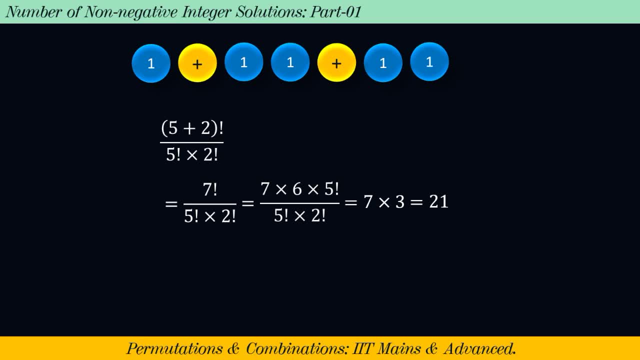 That is, there are twenty-one ordered triplets are there whose sum is five. Let us get some feel. what have we done so far? This sequence represents x is equal to zero, y is equal to two and z is equal to three. 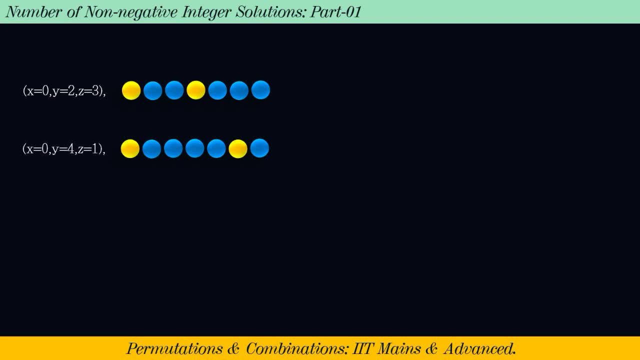 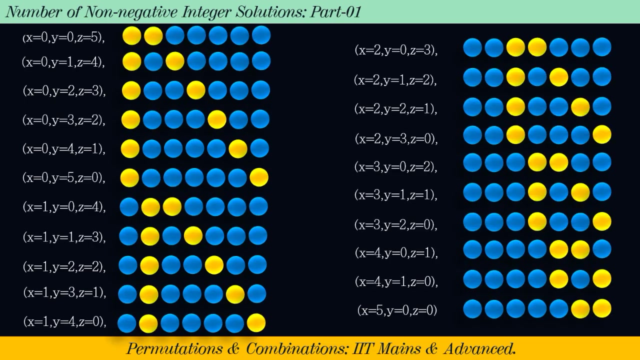 And this one x is equal to zero, y is equal to four and z is equal to one. And this one x is equal to one, y is equal to two, z is equal to two. Here is all possible arrangements. 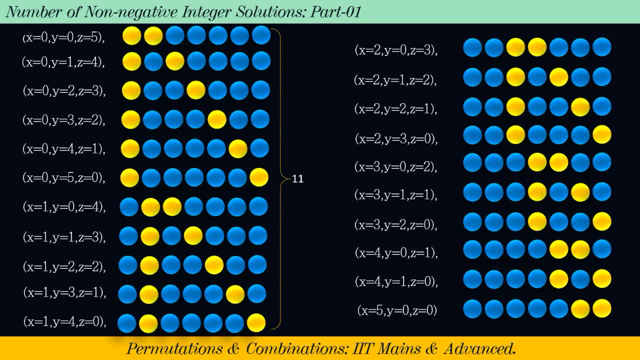 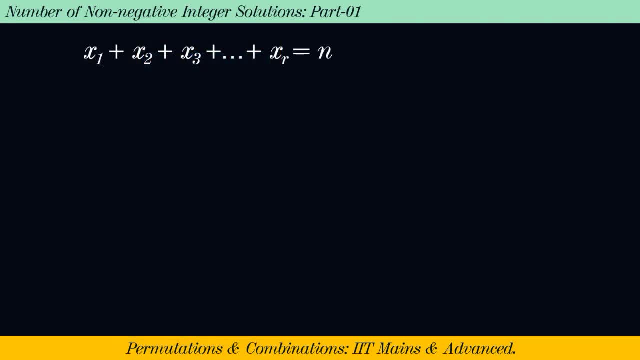 There are eleven on left-hand side and ten on right-hand side. Now no more wait for main question. In previous example we had taken five blue balls because of sum of x, y and z was five, And we have also taken two yellow colored balls because of two signs of addition. 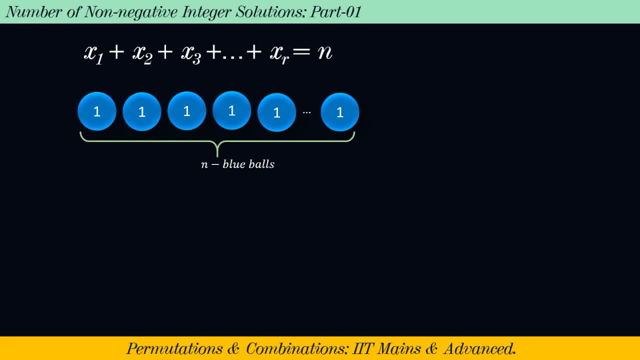 In this situation, we will take n blue colored balls, because sum of x1, x2, x3, all the way up to xr is equal to n, And we will take r minus one yellow colored balls, which is equal to number of positive signs. 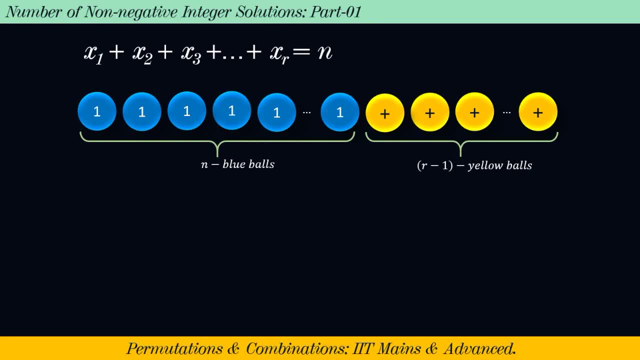 Now we have to arrange a total of n plus r minus one balls, out of which n are of one kind that is blue colored, And r minus one are of another kind that is yellow colored. So the total number of arrangement is equal to. 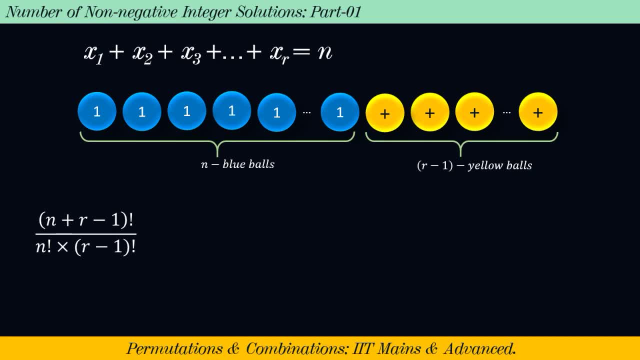 n plus r minus one factorial, divided by n factorial times r minus one factorial. So these many non-negative integer solutions are possible for above equation. Furthermore, we can write n factorial as difference of n plus r minus one and r minus one to get our result in formal notation, which is n plus r minus one, c r minus one.